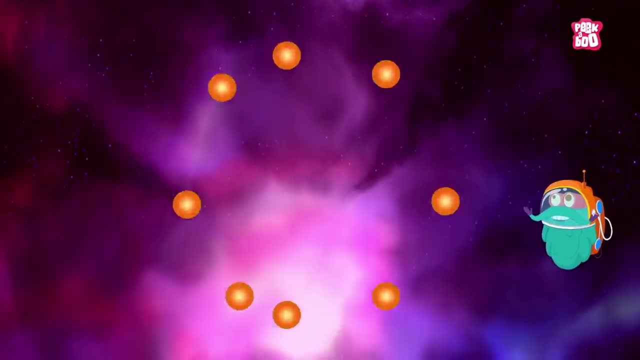 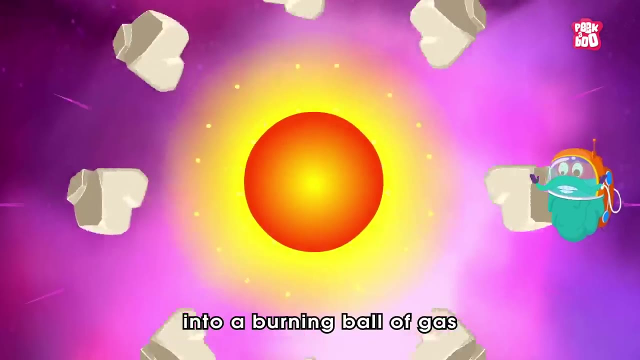 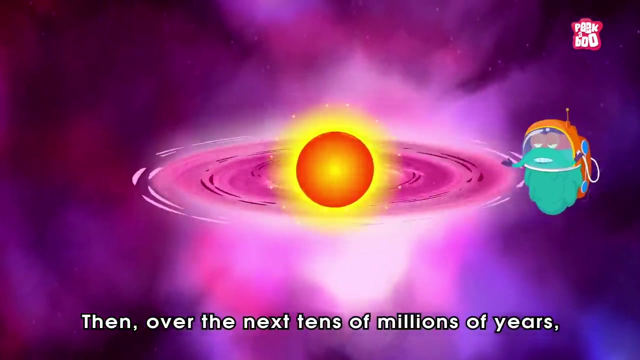 And in the center of this disk formation the material continued to clump together as the matter condensed into a burning ball of gas to form a protostar. Then, over the next tens of millions of years, the temperature and pressure of the material inside increased. 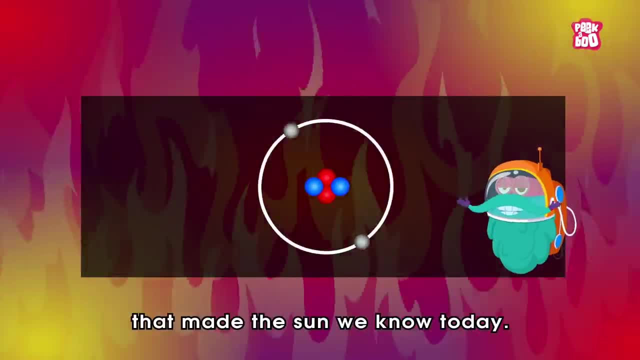 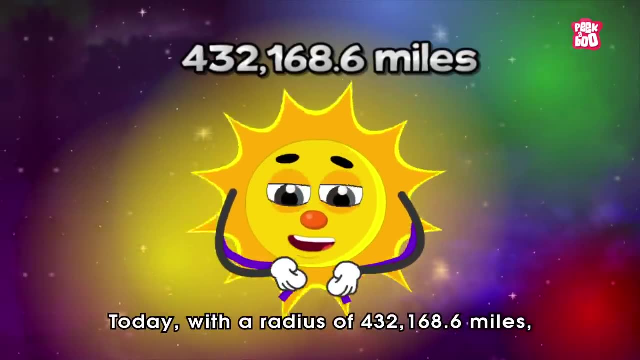 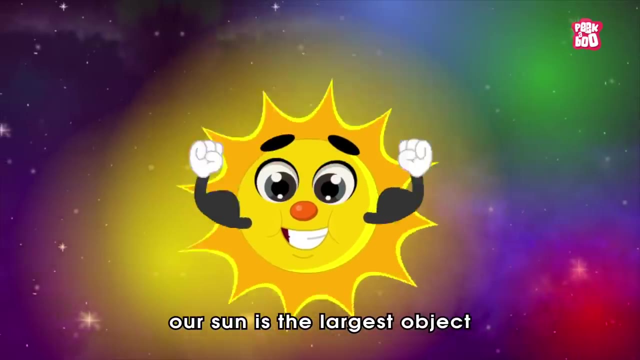 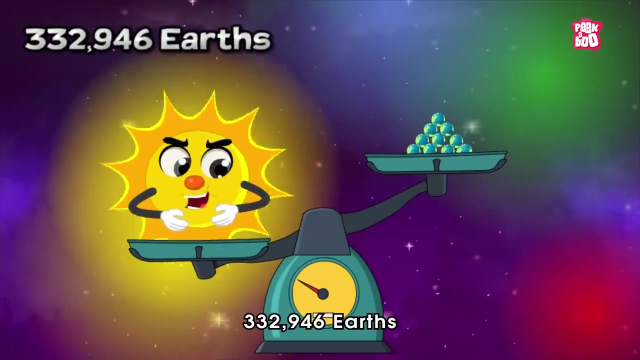 jump-starting the fusion of hydrogen that made the sun we know today. Today, with a radius of 4,32,000 meters, our sun is the largest object in our solar system. It is so big that it would take 3,32,946 Earths to match the mass of the sun. 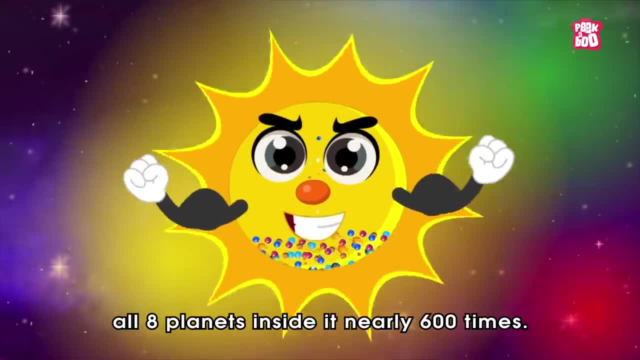 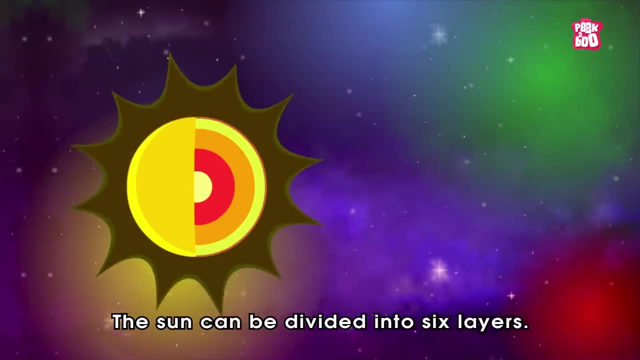 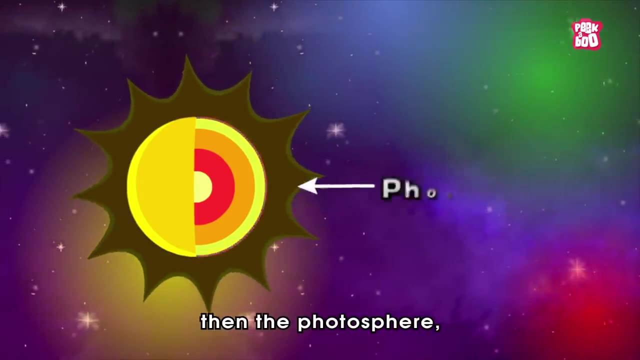 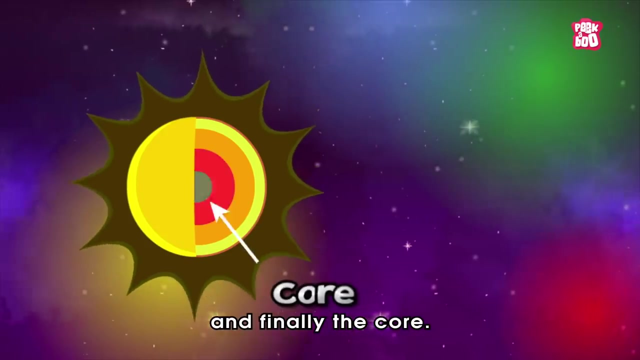 and can fit all eight planets inside it. nearly 600 times The sun can be divided into six layers, Starting from the corona. next comes the chromosphere, then the photosphere, followed by the convective zone, radiative zone and finally the core. 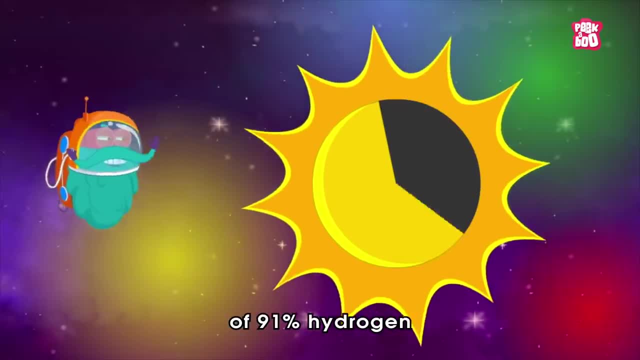 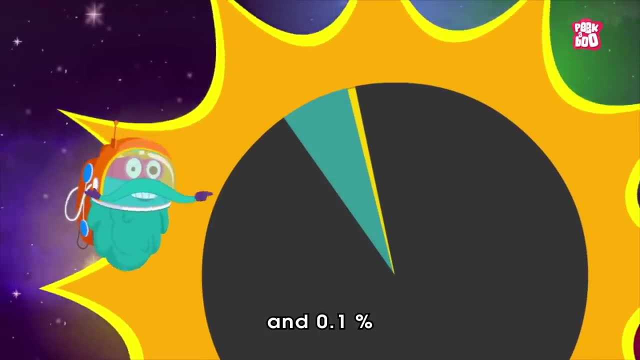 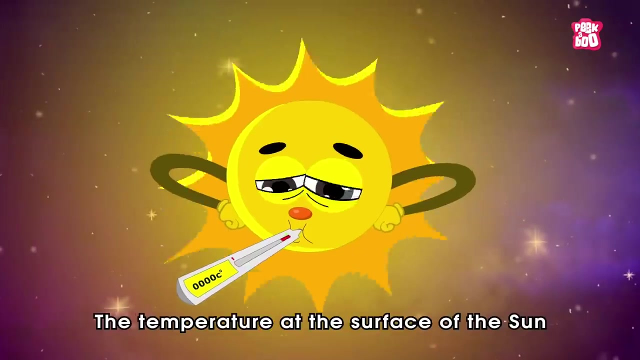 In terms of atom count, the sun is made up of 91% hydrogen that acts as its fuel- 8.9% helium and 0.1% heavier elements like nitrogen and carbon. The temperature at the surface of the sun is about 5,600 Celsius. 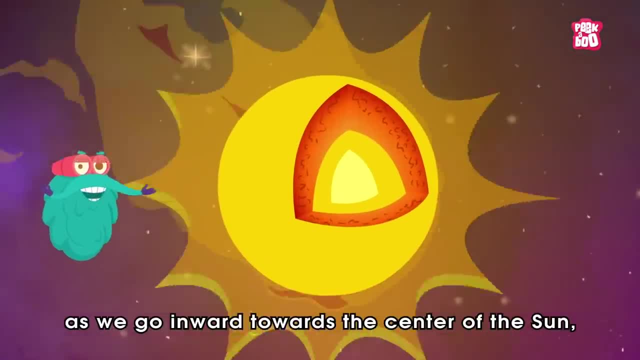 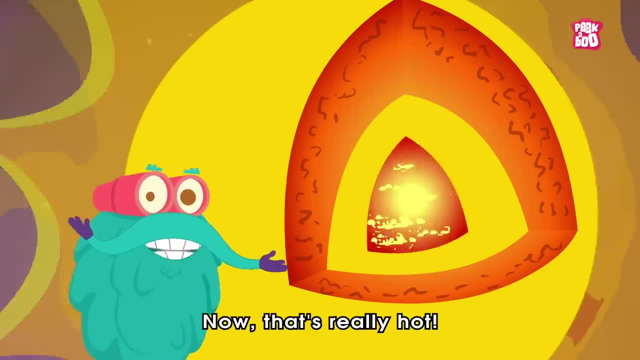 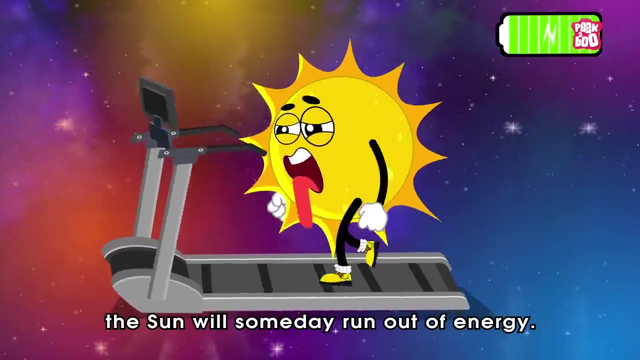 which rises as we go inward towards the center of the sun, where it reaches around 15 million Celsius. Now that's really hot. But here's a thing, my friends: like old stars, the sun will someday run out of energy. Yes, 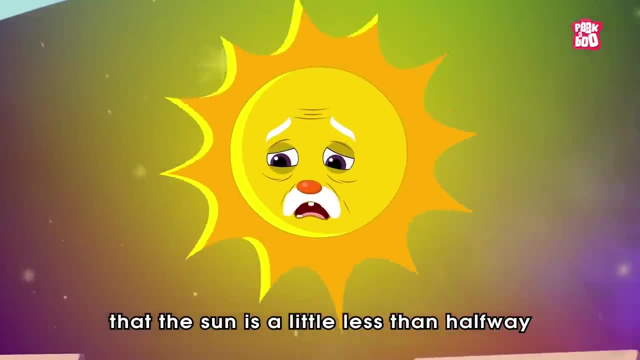 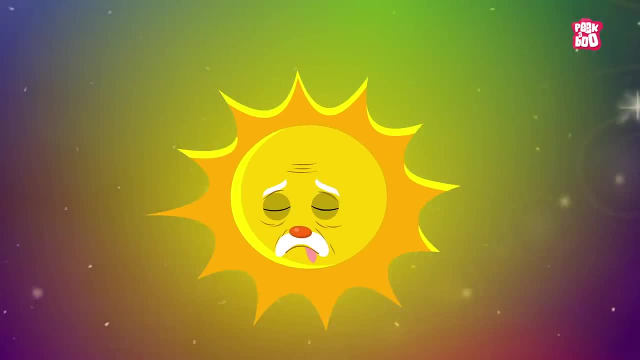 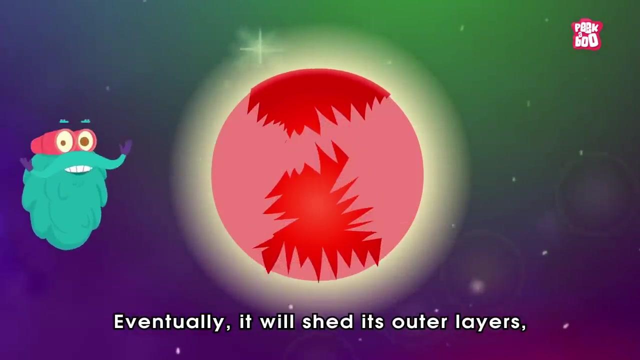 Scientists predict that the sun is a little less than halfway through its lifetime and will last another 6.5 billion years. After that it will swell to become a red giant. Eventually it will shed its outer layers and the remaining core will collapse to become a white dwarf.